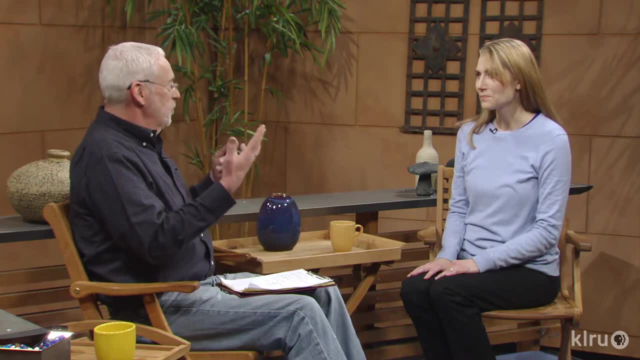 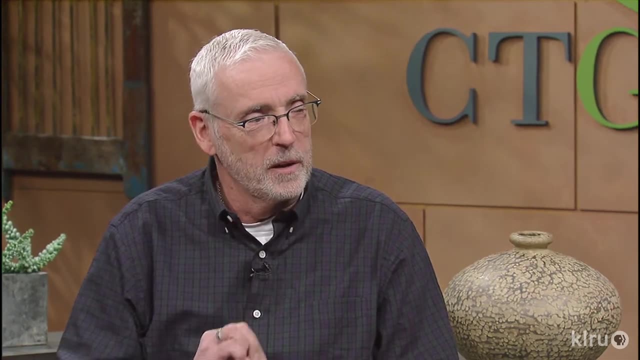 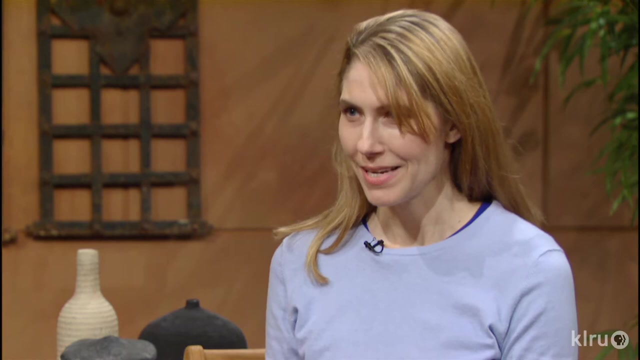 do soil testing and we've heard, you know, all sorts of ideas about soil testing in the past, but you have a specific target in mind here: to look for some of these kind of contaminants, right, Right, well, we provide, at an annual event, the soil. 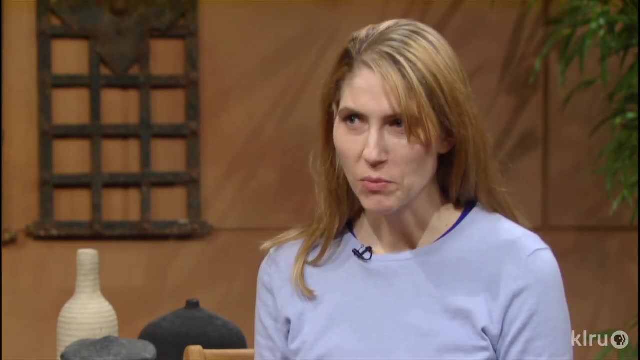 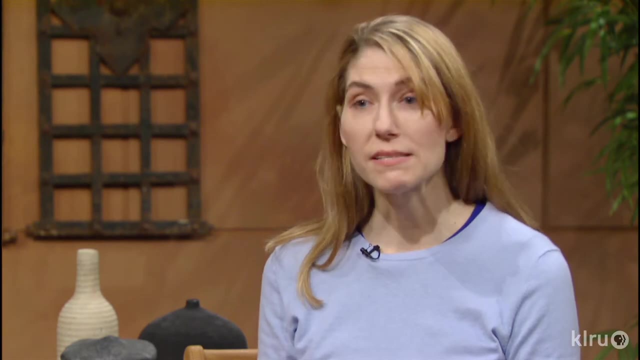 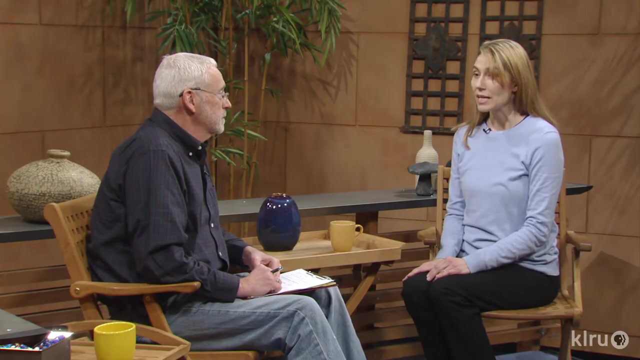 kitchen. we provide free testing for heavy metals and we also do soil nutrient testing and the reason being for the metals is that the heavy metals is that people have contamination or might have contamination and they don't realize it's there, and that could be from lead-based paint on their buildings or 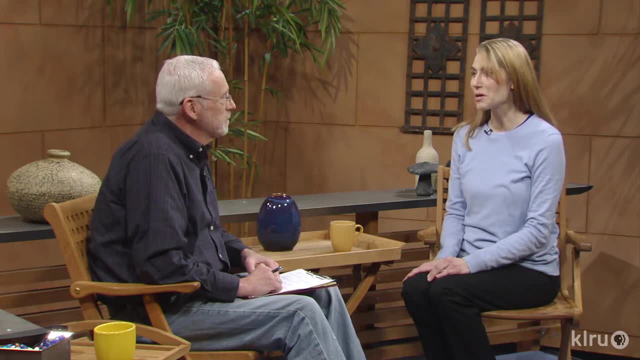 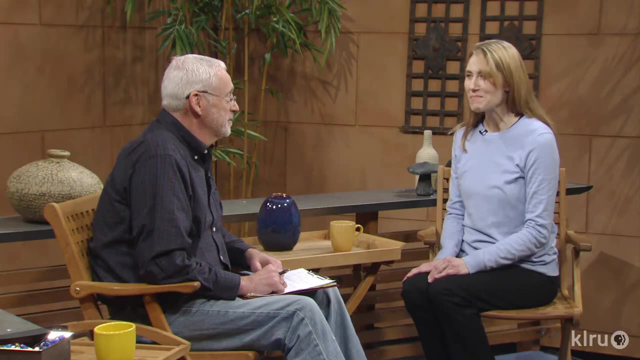 there could have been treated lumber in your backyard from your deck, or a playscape Asbestos siding that's sloughed off or something like that, But that wouldn't show up as heavy metals. Okay, there are a lot of different potential things. Sure, and if property was historically farmland pesticide use, it typically had arsenic in it. Yeah So, and if you're near a busy road, then lead-based gasoline- leaded gasoline used to be an issue, but the lead is pervasive. it is still there. 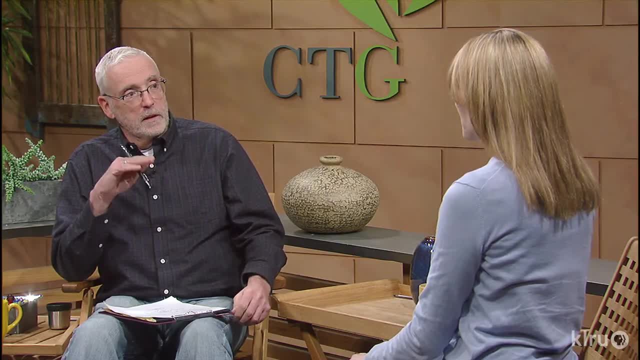 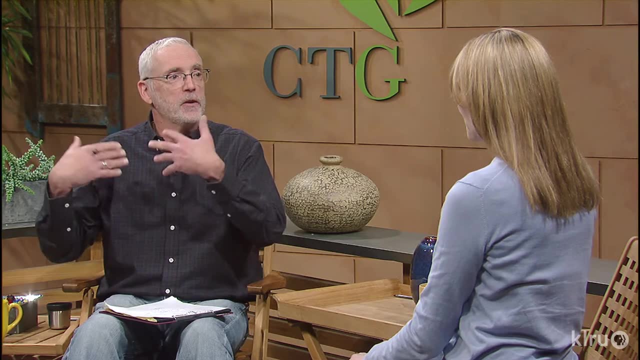 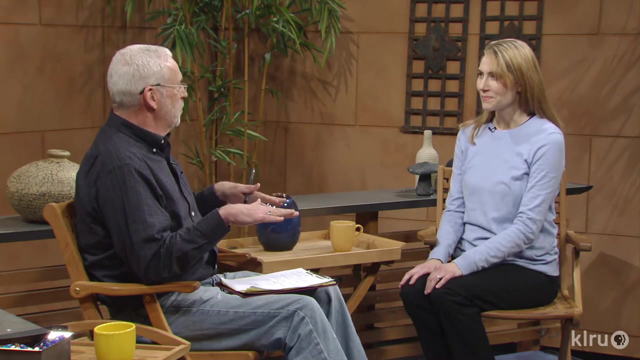 Wow, and you know that's something for people to realize that I certainly was unaware. I thought that if you were kind to the soil for year after year and you added organic amendments and were really working the soil, that would dissipate problems. You wouldn't face things like lead contamination. but 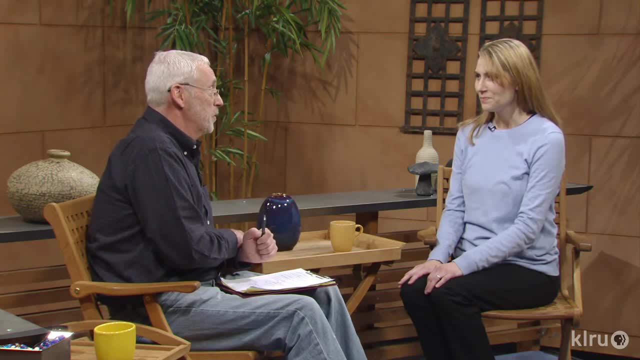 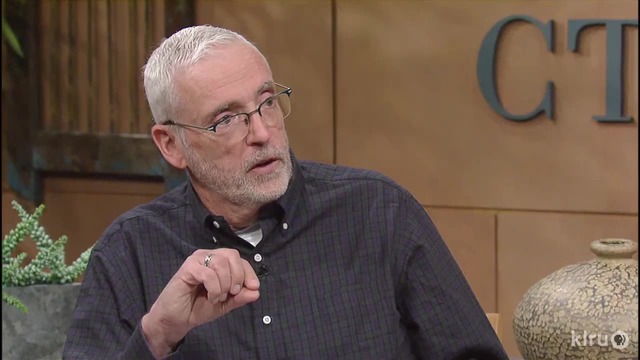 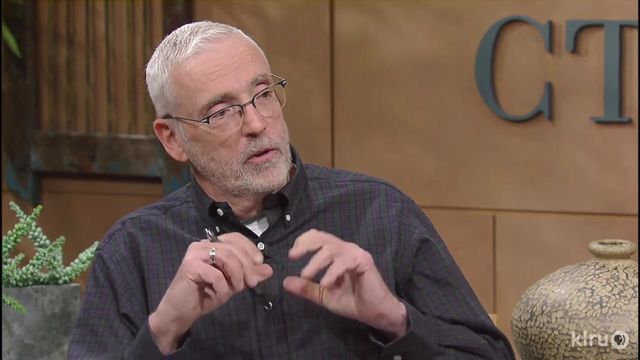 what you were telling me is that lead persists- correct, It does. It will still be there, Okay, so this is important news for home gardeners, especially for those who are doing fruit production or vegetable production. right? Should horticultural gardeners- people who are just doing landscaping- be concerned Are 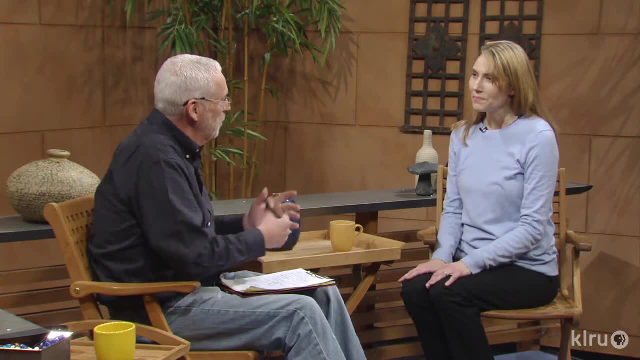 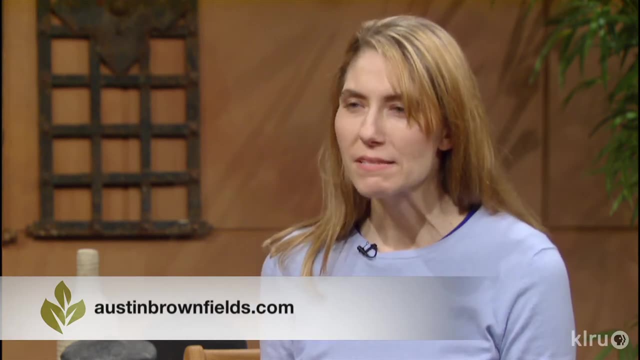 there precautions that they would need to take if the tests come back. Sure, we have that on our website at austinbrownfieldscom, but it's best practices because it isn't so much just well if it's just ornamental plants, but vegetables. don't really take up- lead, for example, very easily, but other things like cadmium they're more prone to taking it up. but that doesn't mean you're not exposed, because people eat root vegetables that they don't necessarily peel, or leafy vegetables where it's really easy for some dust to get stuck. 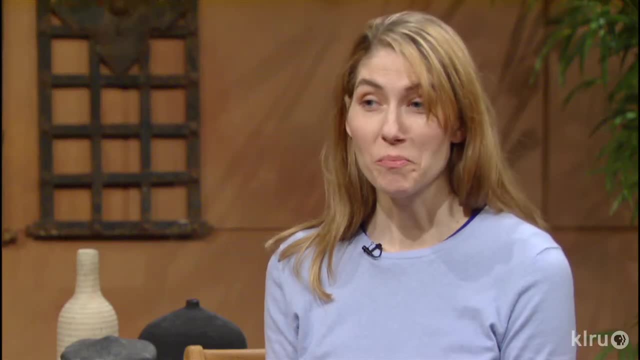 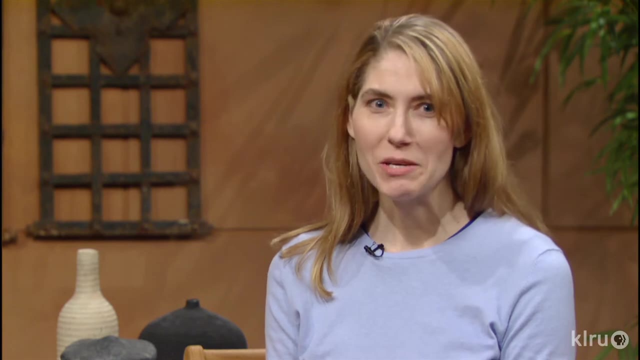 in, or it gets on your clothes or on your pet that goes outside And comes back in your house and then you have dust, Okay So, and it's easy for small children to be out in the yard. and where do kids put their fingers In their mouths? 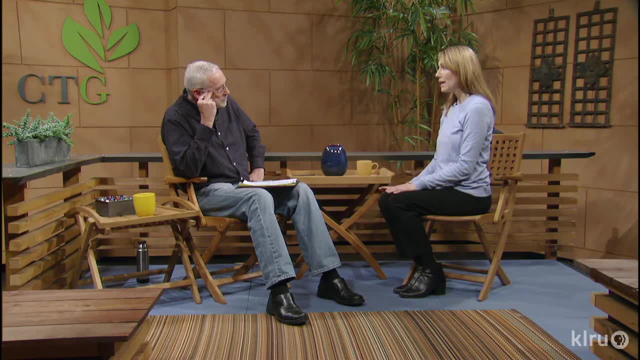 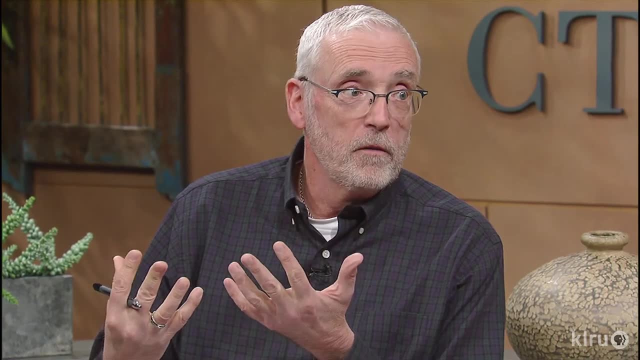 Okay, So it's easier to be exposed to the lead in your soil than just through eating your fruit or vegetables? Is this really a question of helping people just be aware of potential dangers, or are there remediations or steps that they could actually take to help? 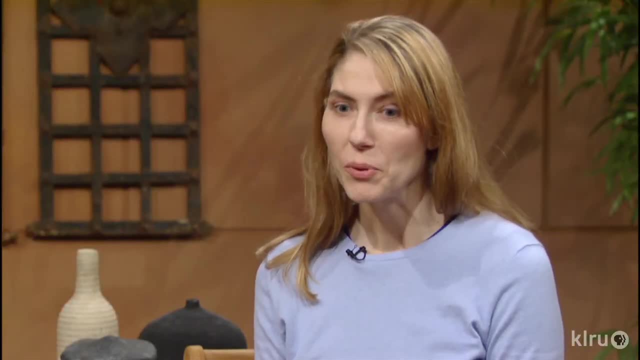 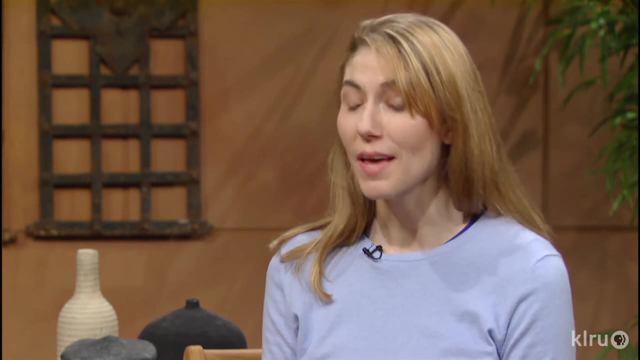 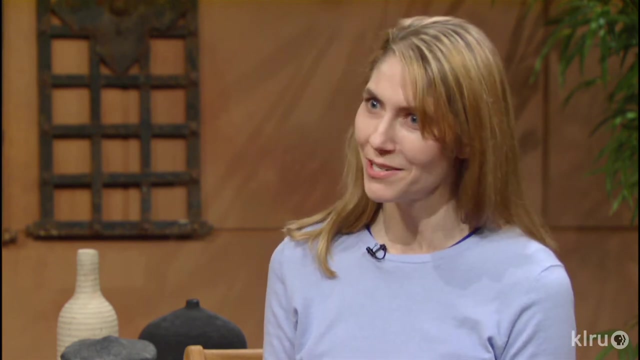 There are steps such as adding compost or putting down paving stones to step on or doing raised beds and just making sure- I mean the things that make sense- wearing gloves, making sure that you're not tracking in dust into your house or soil, and again, that's listed on our 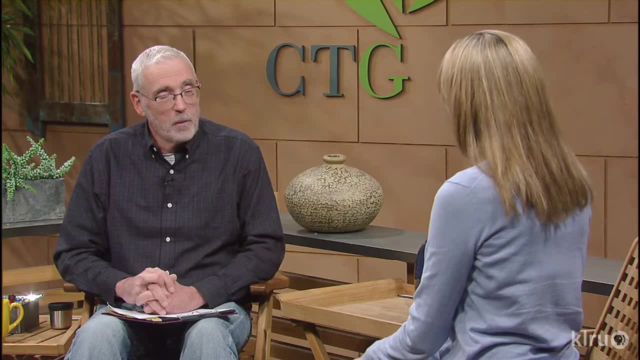 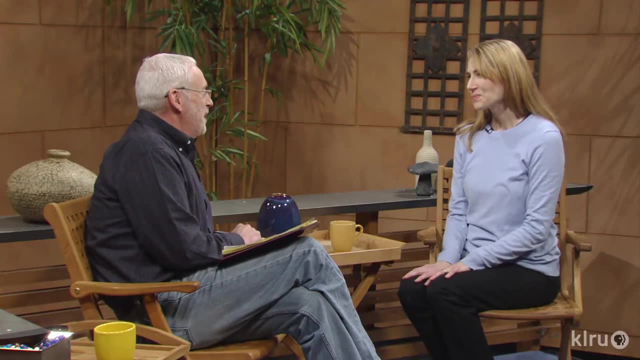 website, But just common sense kind of items. Well, that's good to know that once contaminated doesn't mean permanent, that you need to wear a hazmat suit. A hazmat suit out into the backyard probably would not be the most popular thing to do. 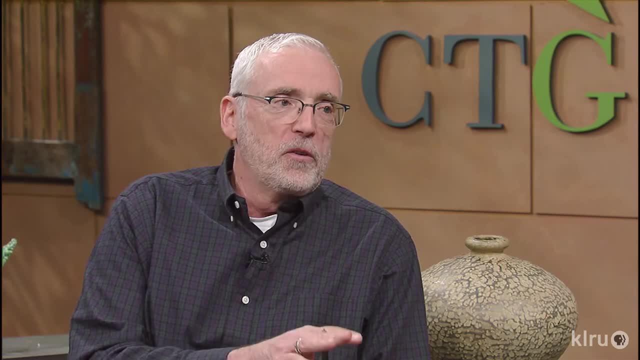 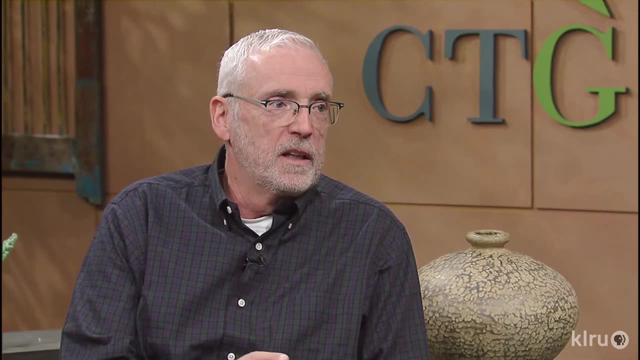 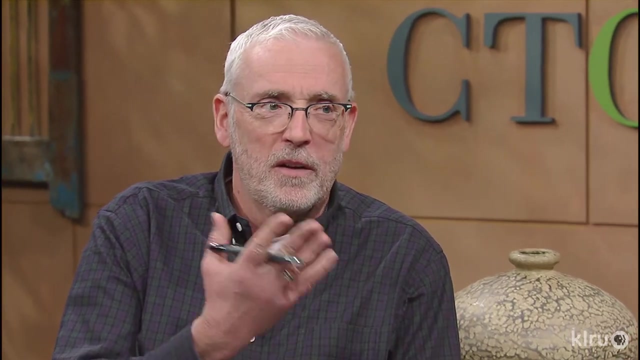 So let's talk a little bit about how you're testing the soils and again explicitly what kinds of things pop up when you do one of these kinds of tests. You mentioned lead and cadmium. I'm not too familiar with what the dangers of cadmium are, but Kidney disease. You could stop it. You could stop there, I'm convinced. Okay, we need to test for cadmium, but what are some of the other things that are common contaminants in the soil Other than arsenic, lead, barium, cadmium, zinc, chromium, mercury? 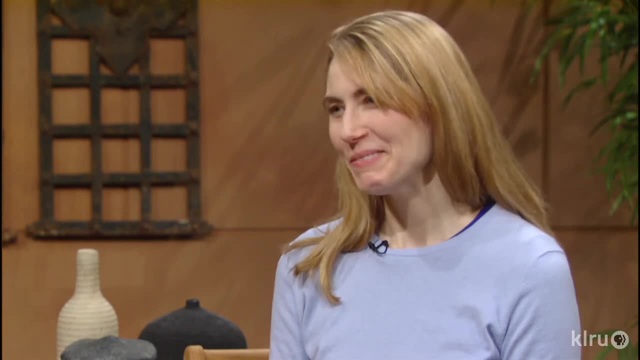 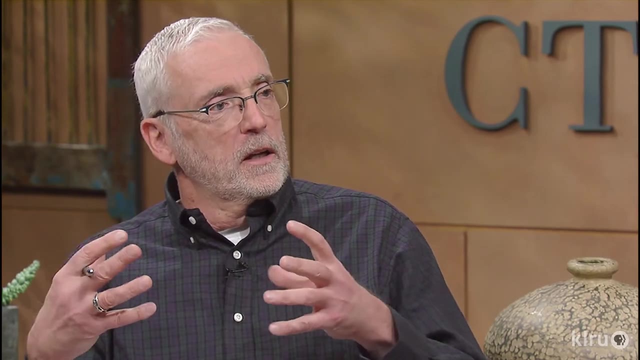 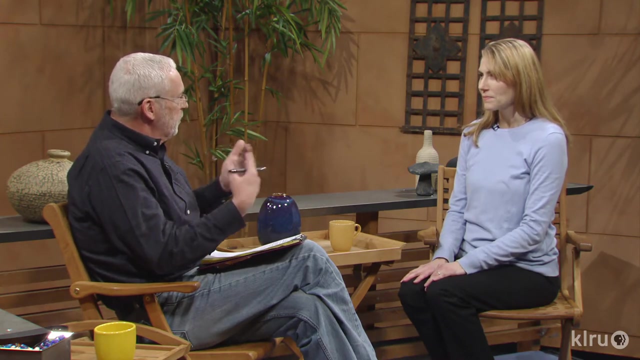 Wow, Okay, A whole host of stuff, Sure, Okay. And should people be particularly concerned, if you know, if they live in a like in like the central city as opposed to new suburbs, or what would be the difference between those? kinds of scenarios. Well, really, it's hard to know what your property could have been before. It could have been an unofficial dumping ground that you didn't know about before it was developed. It could have been farmland that pesticide use. it could have had a cattle dip if it. 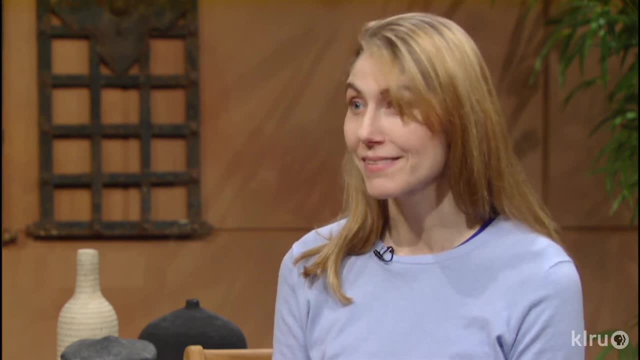 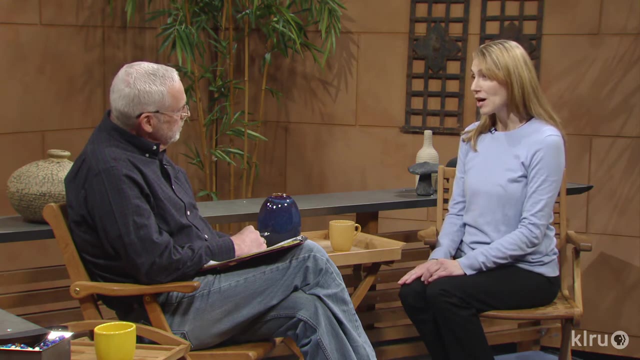 was farmland, which that was arsenic based. Okay, Way back in the day, Mm-hmm. And even if it is a residential area now, it doesn't mean that 50,, 80 years ago it still was. 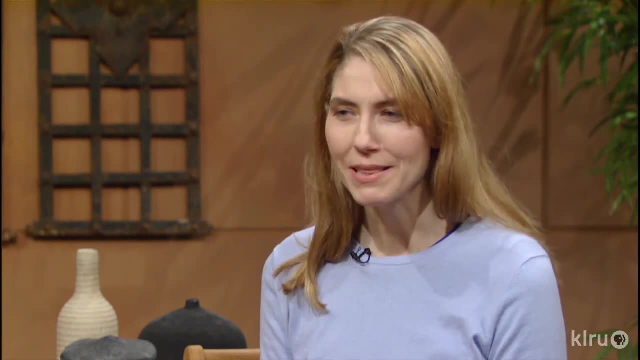 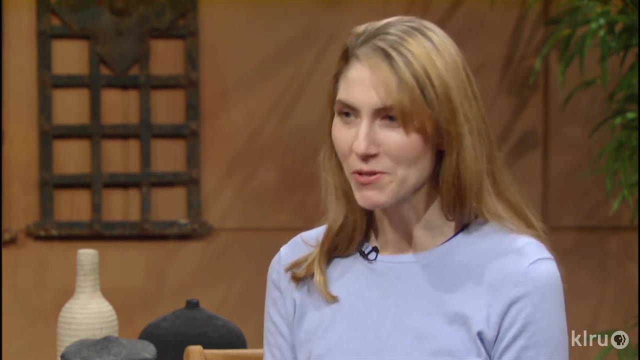 Right, And if you have a new house, it doesn't mean that there wasn't an old house there before- with lead-based paint, Mm-hmm, Or treated lumber. So it's just good to know what you're starting with. and that's the same with soil nutrients. 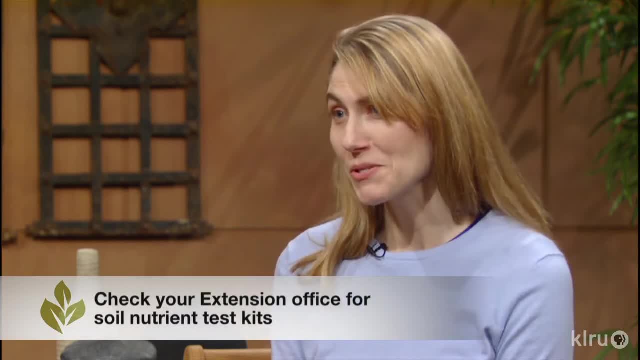 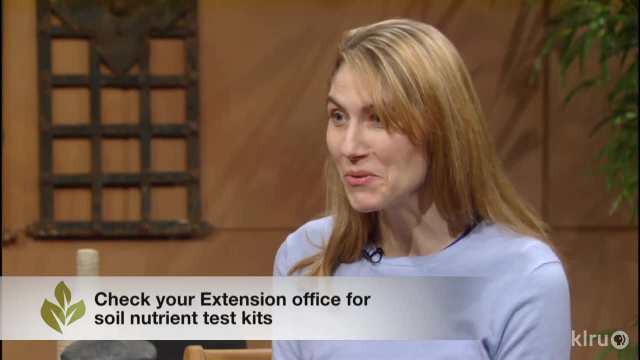 Mm-hmm, Because even if you say, well, adding compost is a good idea, or if you're not adding fertilizer, but Mm-hmm If you're buying plants that live there before, add a lot of nutrients. 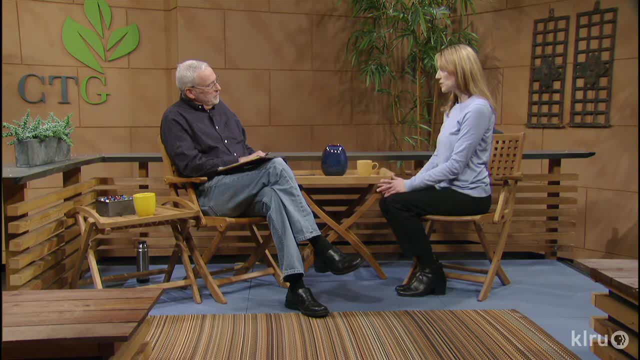 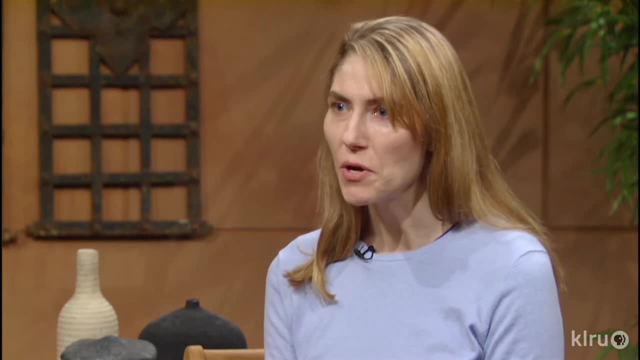 Right, Or did they add a lot of fertilizer, Mm-hmm? It's just good to know where you're starting at, and we also get the pH results. Okay, And so that at least lets you know where you're starting from. Mm-hmm. The soil around Austin, for example, is highly alkaline, Yeah. So if you're buying plants that like more neutral soil, Yeah, Then you're not going to be successful, Or acidic-loving plants- they Azalea's fantastic. 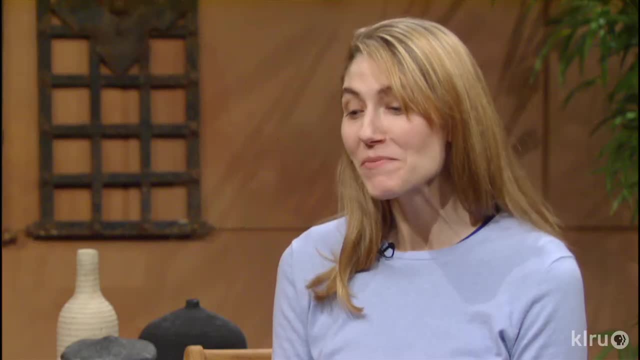 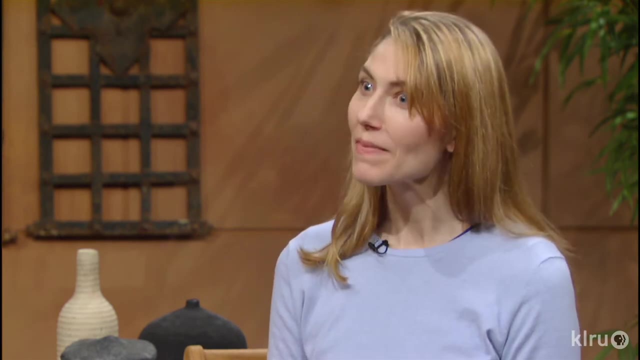 Azalea's bad idea, Then you're just not going to be successful. and some people think, oh, my plant is not being very successful, and they think fertilize, fertilize, fertilize, and that's not helpful. 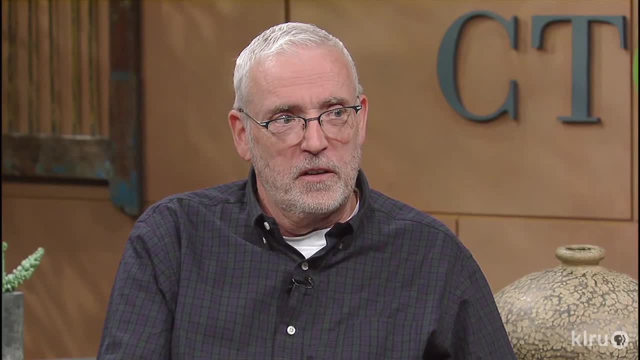 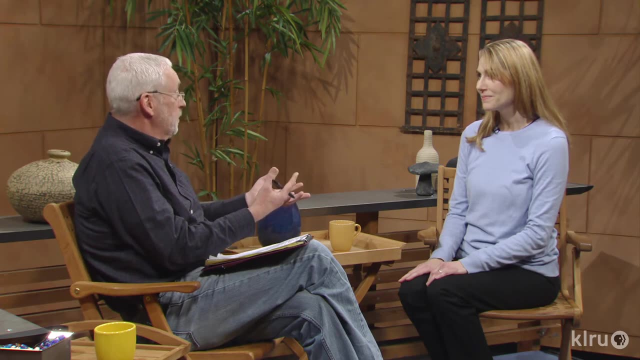 Or that they could actually change the pH, and that's a subject of great interest. Can somebody, by amending the soil, by using something like soil, sulfur, et cetera, can they actually significantly impact the pH level? Yes, you can. 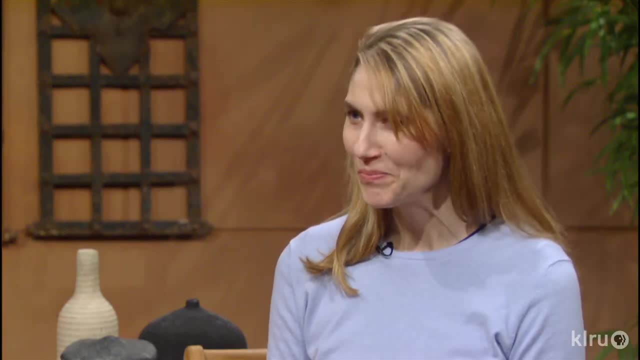 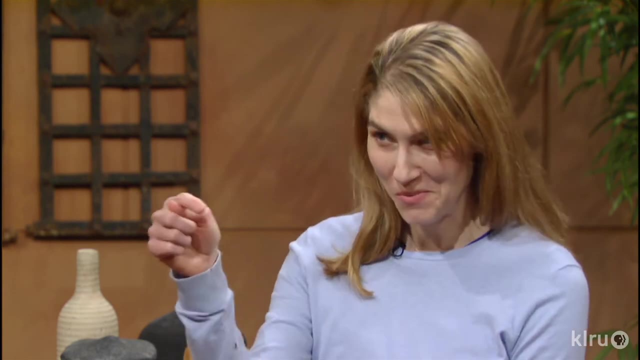 Okay, But you can also add pine needles. Okay, All right, It's harder. I think well, you would know better about this, but isn't it harder to turn it more neutral from alkaline than it is to make it? 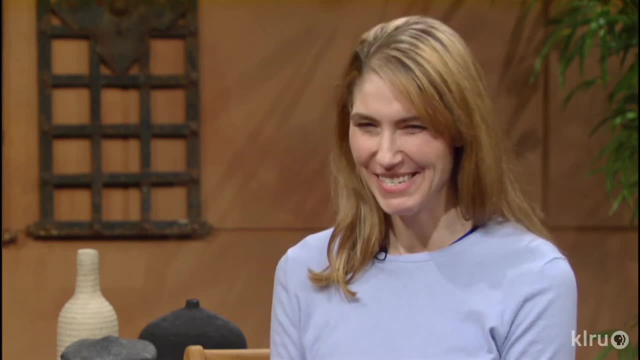 Yes, Yes, Because you can put a lot of lime in your soil much easier than you can move it in the other direction. I don't know anybody who puts lime in their soil in central Texas, to be fair. No, no, no, not in central Texas. 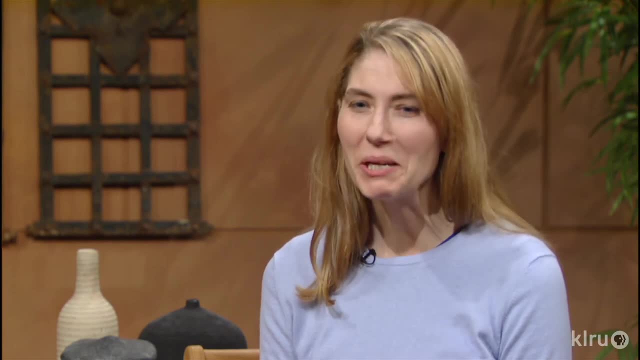 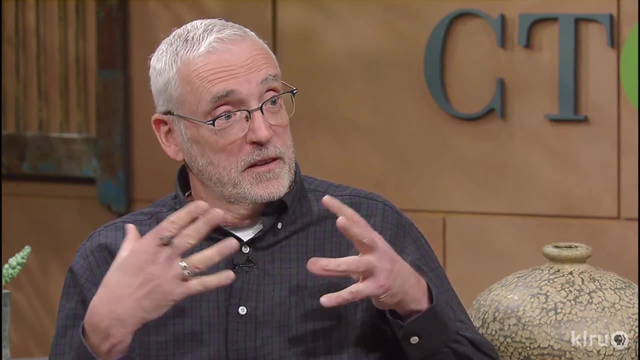 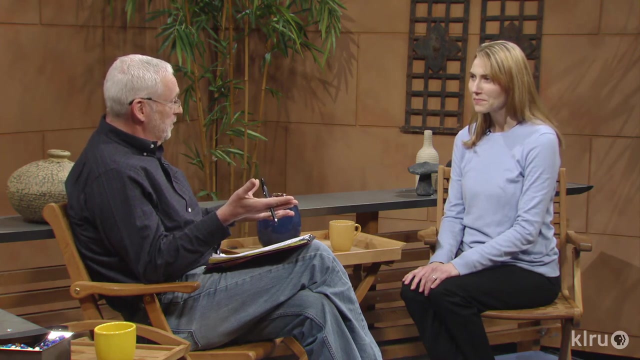 No, But going in the opposite direction is easier than trying to make it more neutral from alkaline. Okay, Right, And I like your suggestion of pine needles and things like that pine bark, you know, Yes, And so I'm hearing soil sulfur can be a successful medium for. Sure, it just might take several years. Yeah, don't expect overnight results. Don't expect overnight results, Right? So, for example, in Austin, and probably many communities around the United States, do this, we do Christmas tree recycling and grinding. Yeah, right, Right, And so you can go and pick up free pine malts, Right, So that is helpful, if you know. hey, I want to move it a little bit and it smells good, So that's a good thing to put in front of your house. 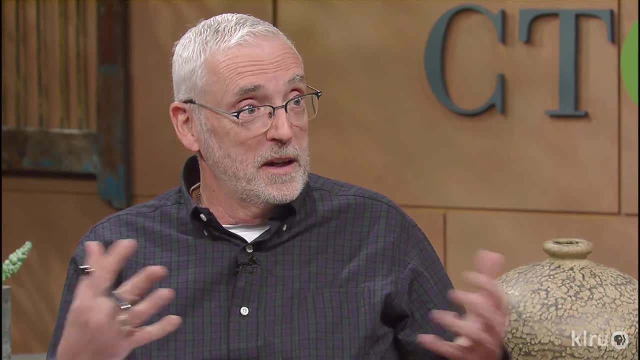 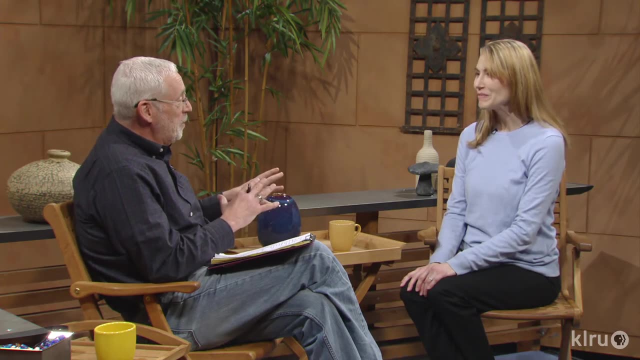 Of course, right, And that's something that Austin led the way on that, but now that's almost nationwide, I think. the Christmas tree recycling: Hopefully everybody's giving that mulch away. A lot of people use it in their parks as well. 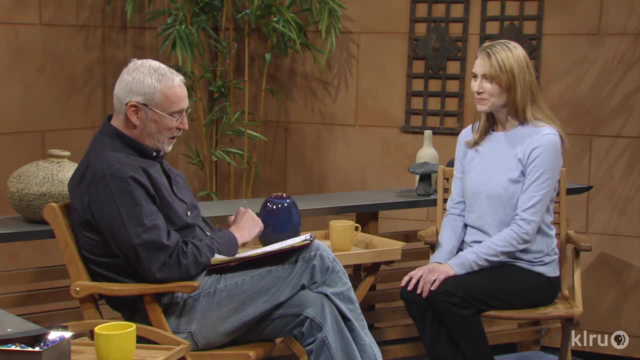 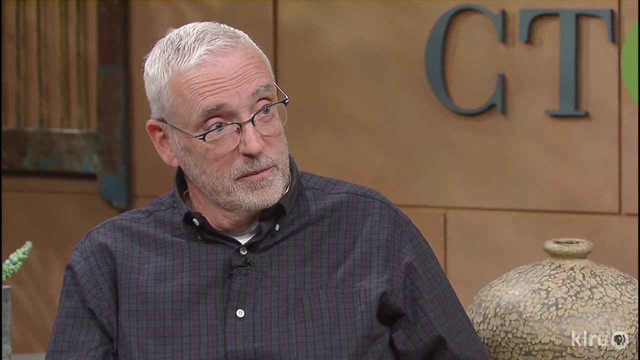 Oh okay, But still great resource available. And there are other great resources out there, Yeah, And there are other great resources that are available through the city of Austin, where you can pick up mulch and things like that as well. So encourage people to do that.